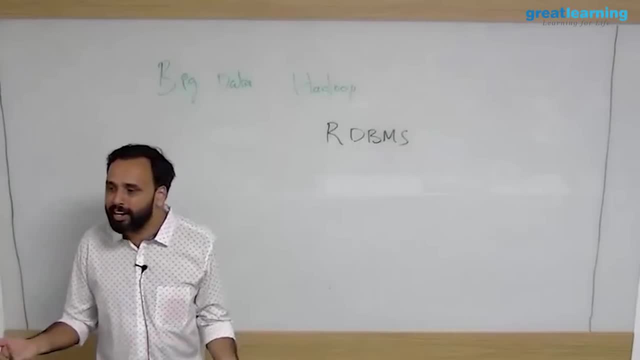 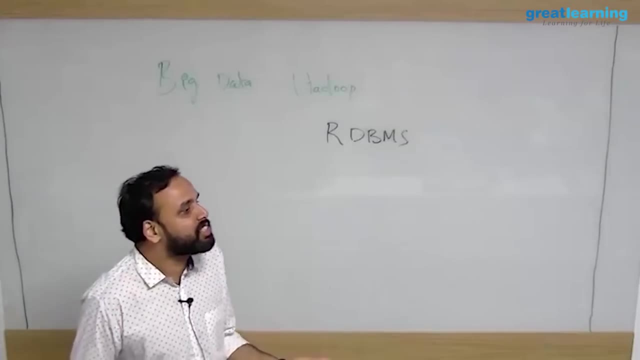 we were using to traditionally store the data. right, and what is an rdbma system? it has a row column format. you have a table, you insert the data. now, if somebody is teaching you rdbms, they will say that, well, rdbms is great, it can store everything you know. that's all fine. but unless 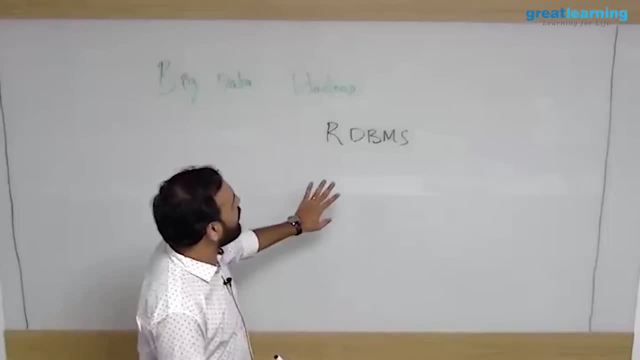 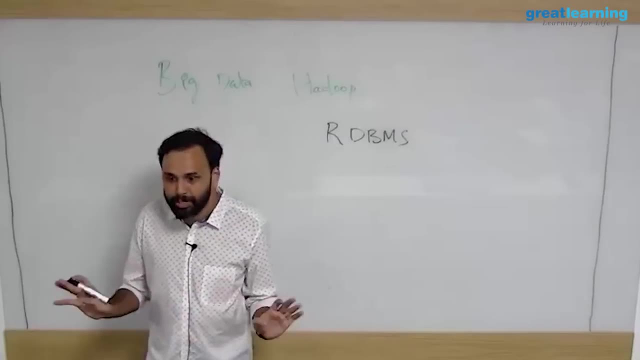 your data starts increasing right. so originally rdbms can store everything. i don't have any. i'm not against rdbms or something, even for transactional management. we use rdbms, there is no doubt about it. mysql oracle: we were using mysql actually. so whatever the customer is, 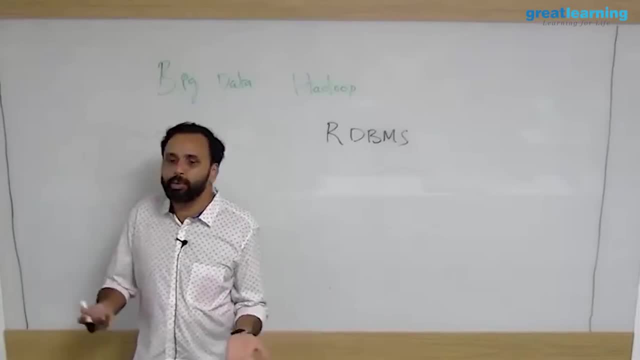 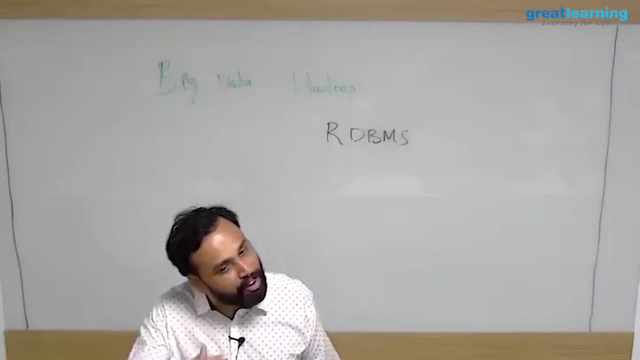 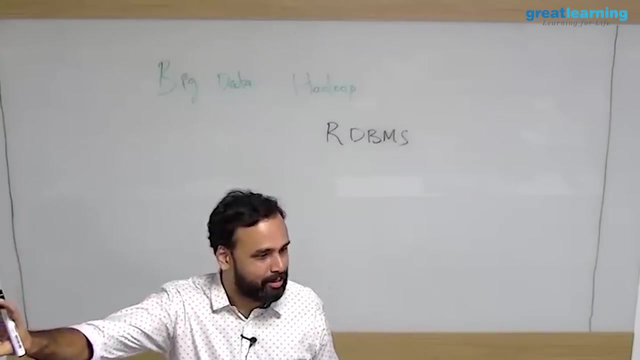 inserting this mysql will capture it. end of the year. you do some processing, you will understand how many items were sold. everybody is happy, happy. this is what was happening in 2005.. fast forward to 2011. i am working with icica bank. icica bank want to migrate to big data platform. so what is? 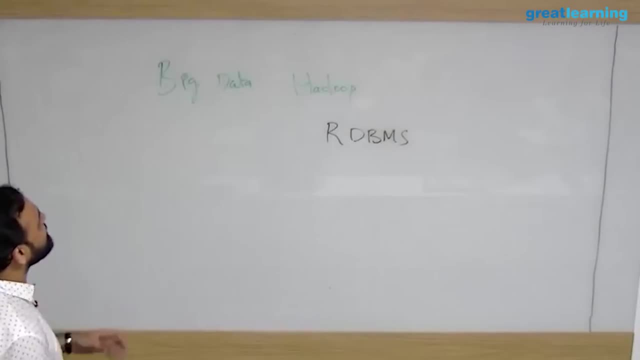 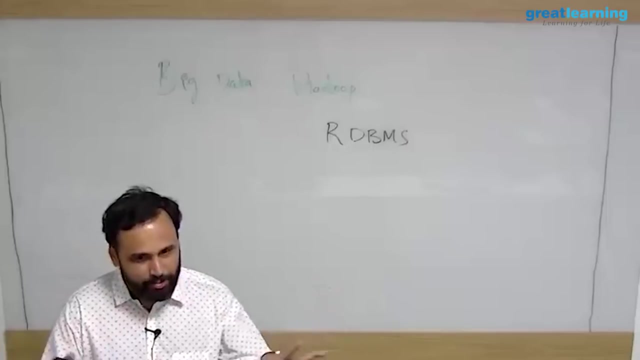 the problem with icica bank, right? so that is the question: why icica bank want to go to big data right now. this example will also help you to understand the it world, right? so for people who are not coming from the it background, they might need to understand how things are working, right. 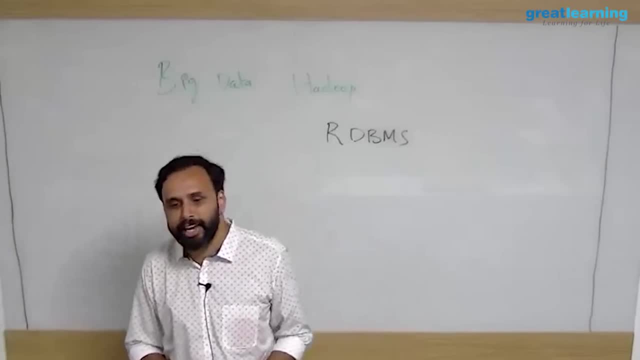 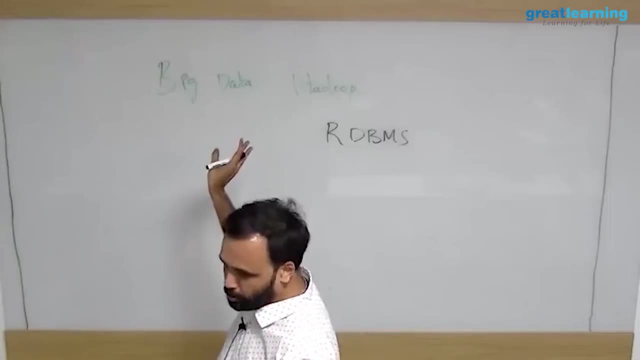 so we we went to icica bank, we spoke with them. we said, hey, what? what do you want? they said: you know what? we are facing a lot of problems. we want to go to big data, we want to go to hadoop. we'll see what is hadoop later. so we asked: what is a big deal? what is your problem? 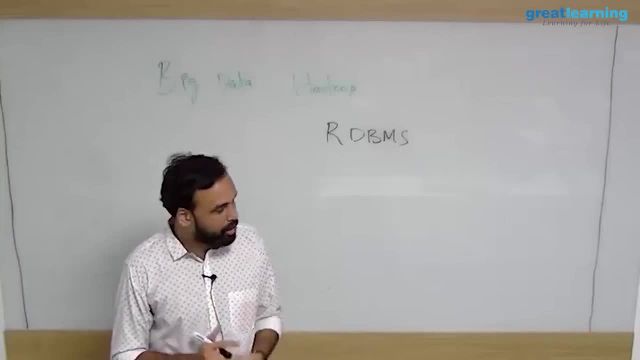 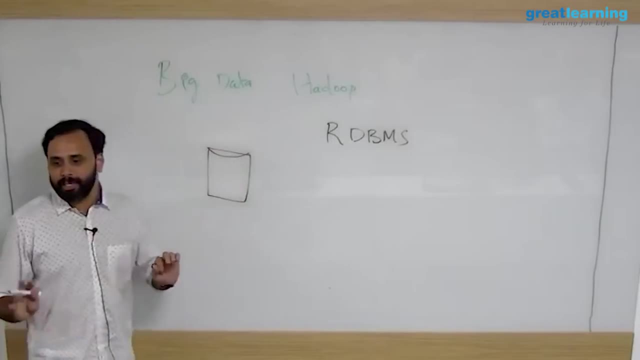 so there were a lot of problems which they were facing. one of the problem is that if you look at this rdbma system- right, your typical rdbma system- what is rdbma system doing? they will store the data in the form of a table right now, if your table size is very, very small. 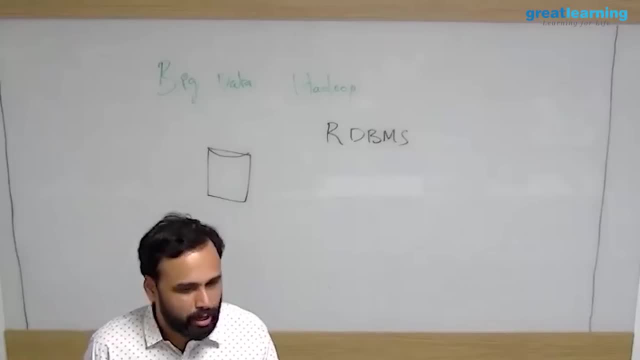 it's not a big deal, even if you look at my sql or if you go to enterprise scale oracle and all you know they can store gigabytes and sometimes up to terabytes of data. but as the size becomes big, so let's say i ask you, okay, you can share the website if you are. that's another big part, if you. 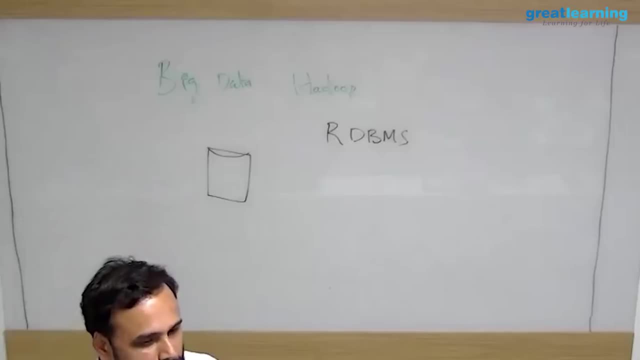 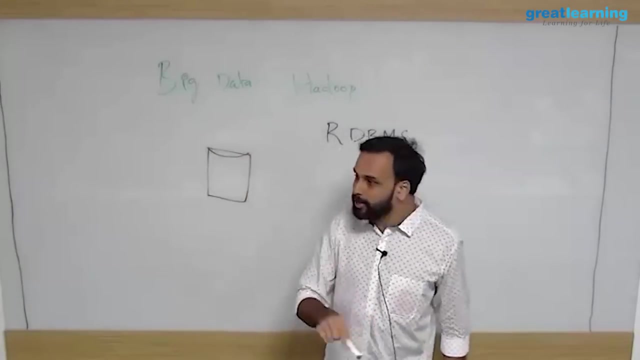 you. You have to store the data in Oracle. The data is keep on increasing every week. You are not ready to migrate anywhere. Oracle- if you talk only about Oracle, they have storage separate and DBMS engine separate. In Oracle. what I can do: I can purchase Oracle and I. 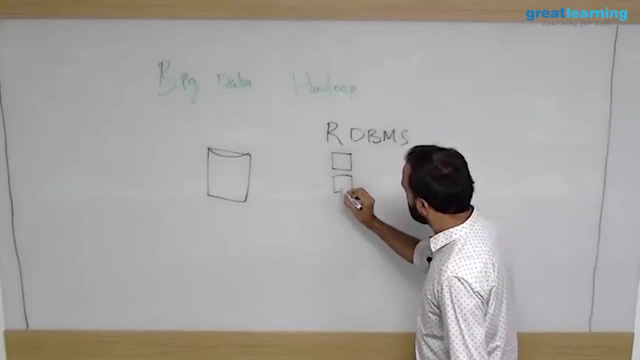 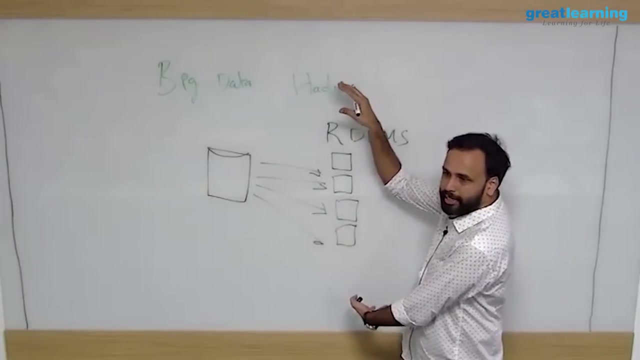 can add storage boxes as many as I want. So these boxes will be in the network, So my database engine will be connecting to them and storing the data, whatever data I am giving. So you can argue saying that I can increase the storage capacity and then Oracle can store. 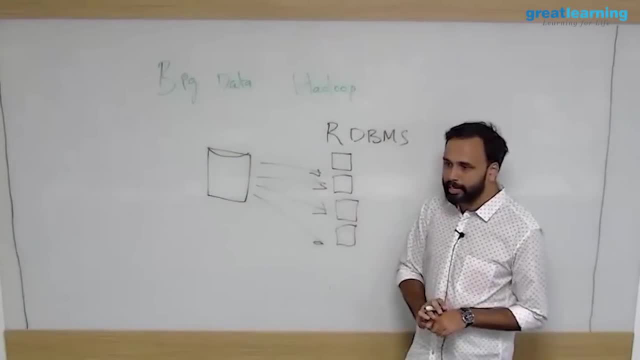 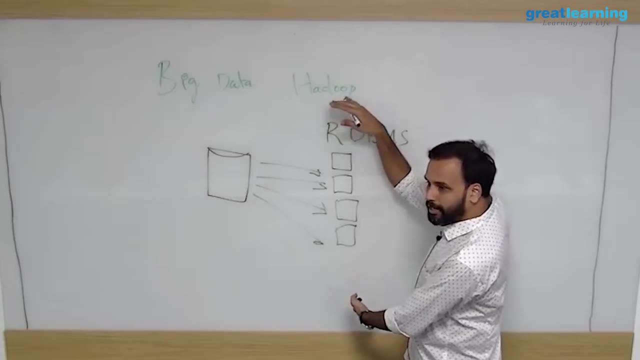 as much data as you want, There is no doubt about it, Right? But there is also a limitation for the storage One problem. Second problem is that as this box increases, the storage in Oracle increases, you have to divide your data. So you are selling iPhone, Let's say. 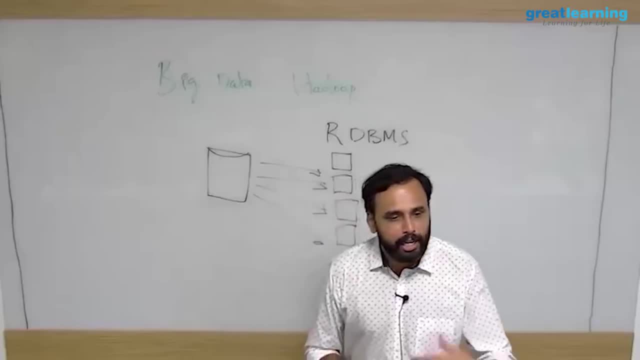 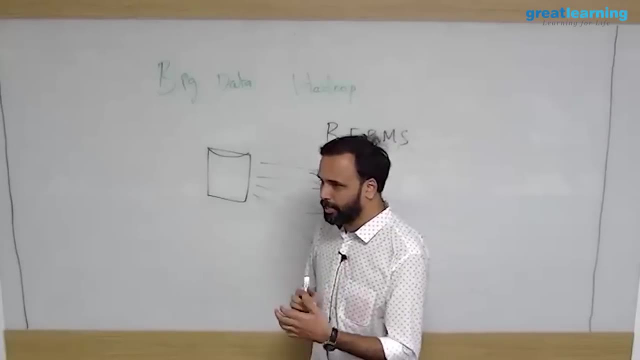 you're working with Apple, Right. So one of the examples- let's say, you're working with Apple, right. So one of the examples is that if you are creating tables to store iPhone data, typically, if you look at the schema and all what we will do is that there will be one table. Okay, There'll be one table. 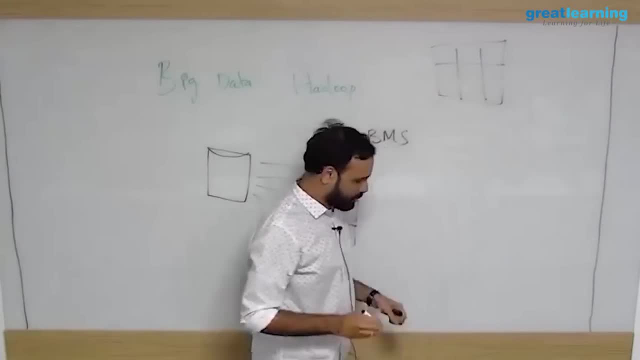 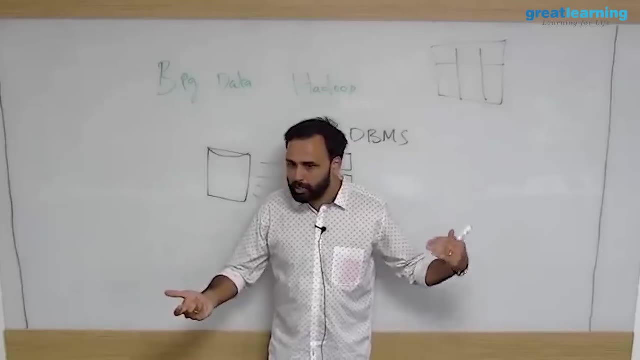 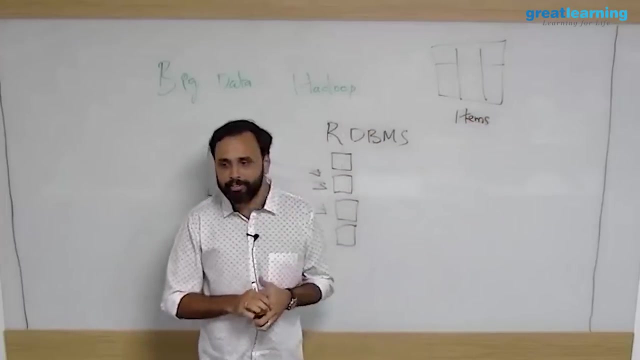 wherein you will be having properties. like you know how many items were purchased, at what rate they were purchased, how many people bought, so on and so forth. So this will be your items table. So in the items table you will have all the data related to the iPhones. 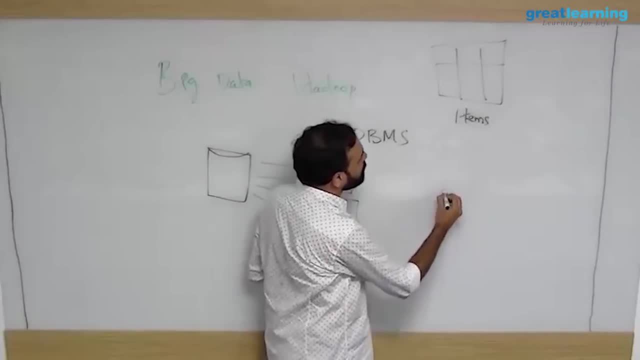 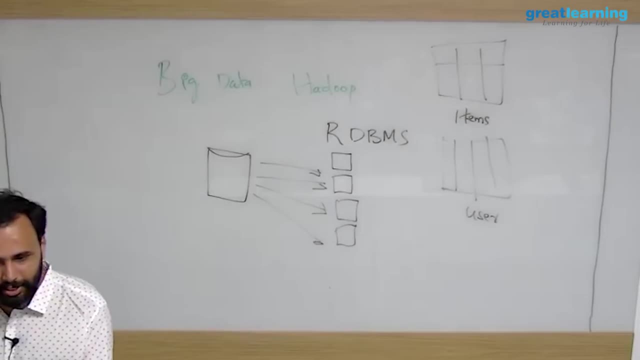 you have. So this will be your items table. So in the items table you will have all the data related to the iPhones you were selling, Right? You will also have another table where there'll be the user data. You will also have the user data. You know what is normalization? 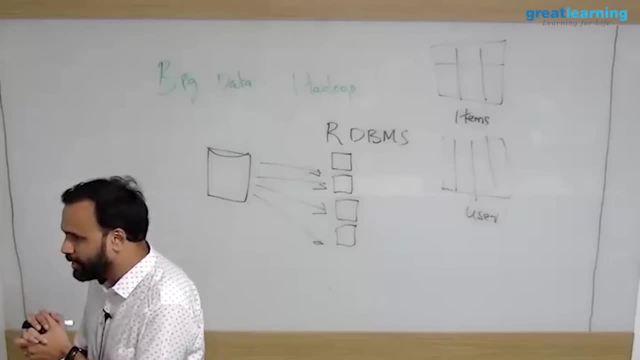 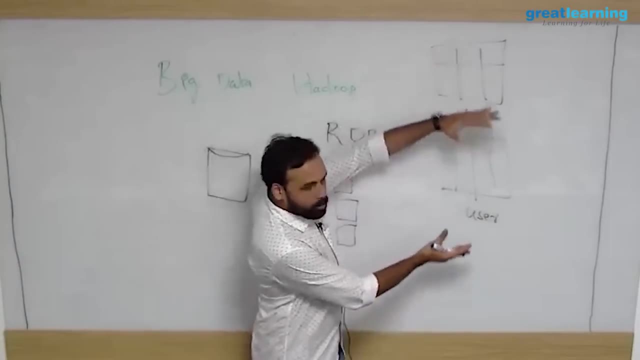 In RDBMS systems in order to avoid duplication of data. what we do is that we normalize the data. We always keep the data in different, different tables. So if I want to get both the data from this, I have to do something called a join query. I fire a join query and 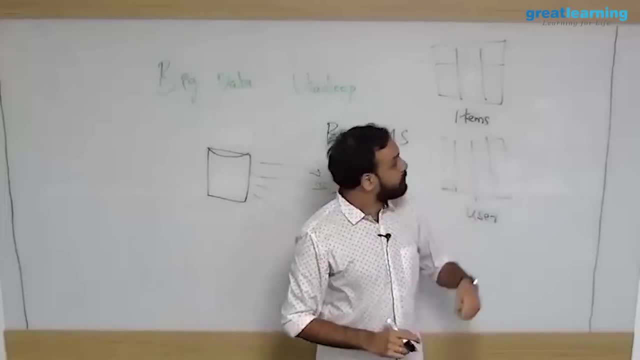 all the data from here will come and join and produce me the output. So if I want to get both the data from here, I have to do something called a join query and all the data from here will come and join and produce me the output. This is good if you're having 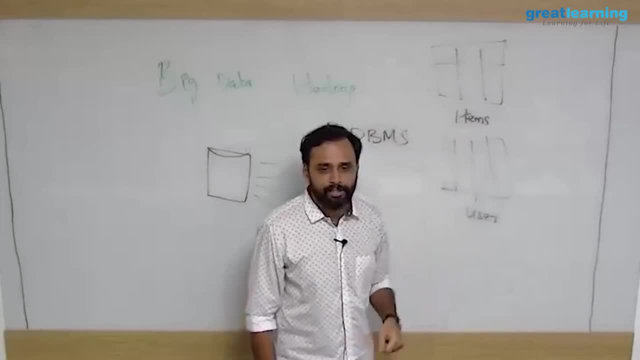 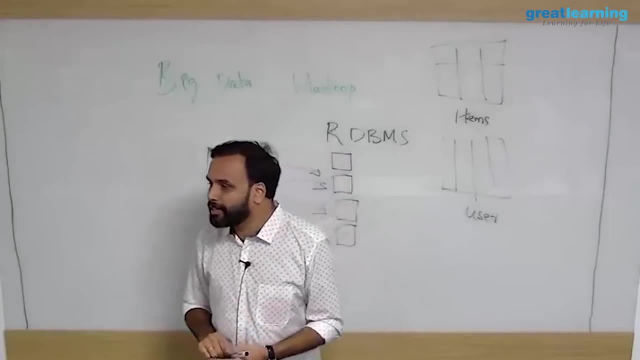 small amount of data. What if you have terabytes of data here and here? My join query will fail Right Or the join query has to wait Now. another point that people say is that if your RDBMS is becoming bigger and bigger, why don't you partition your data? That is, 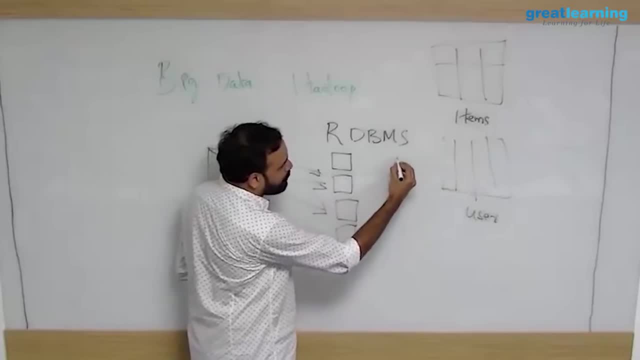 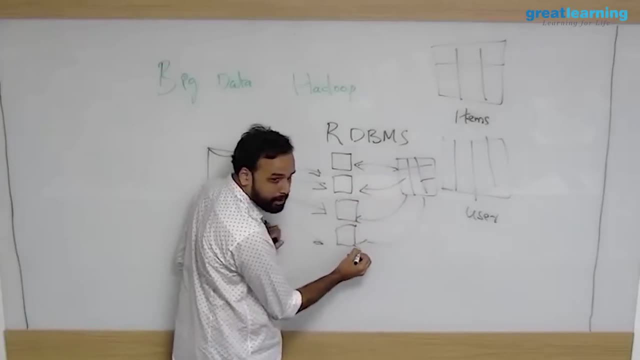 possible. I can have like four boxes, my one table. okay, if this is my table right, it can be logically partitioned and kept on four machines. if it is becoming bigger and bigger, This is possible. There is something called logical partitioning. Look at the iPhone data. 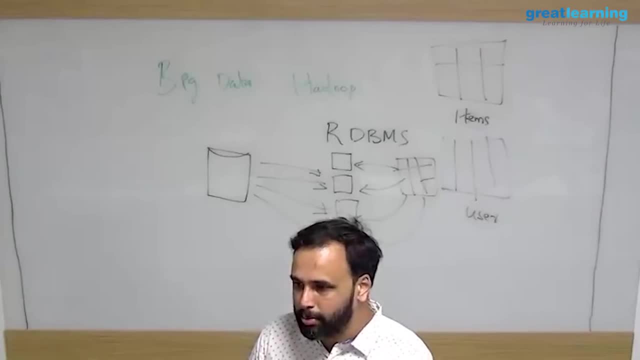 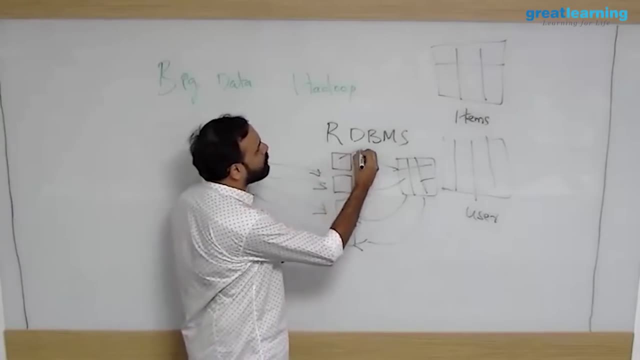 I can say all the data where people from India are buying the iPhone go to this machine. that's called logical partitioning based on the country column. So here I have all the India data where people are buying iPhone. Here I have the US data where people are buying the iPhone. 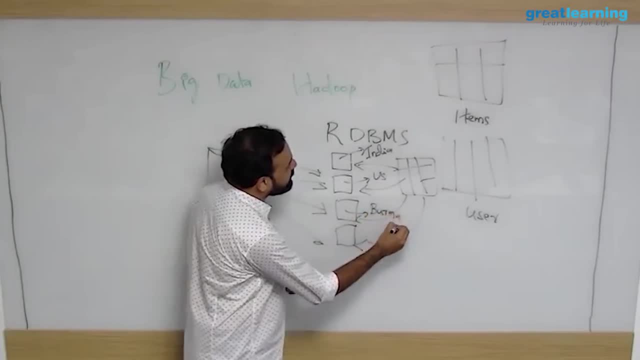 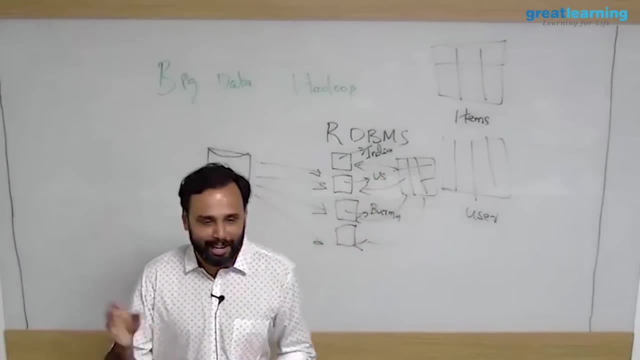 But the problem is here I'll have the Burma data also. India data will be, let's say, two terabyte. China data will be three terabyte. India data will be KBs actually because in Burma I don't think a lot of people are actually. 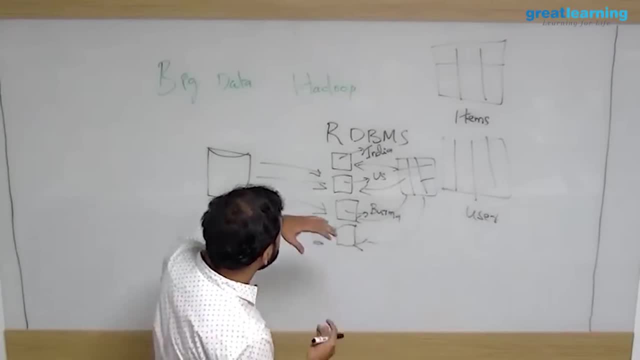 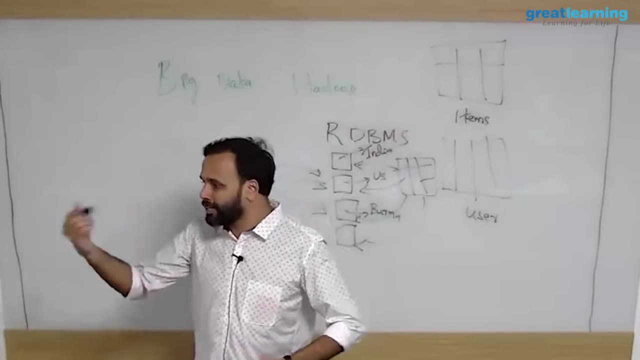 buying iPhone? probably right, Exactly. So the problem is that if a table is becoming so big, okay, I can cluster it. I can take four machines in my RDBMS or data warehousing architecture and I can say: partition the data. Because if a table is so big, if I fire a. 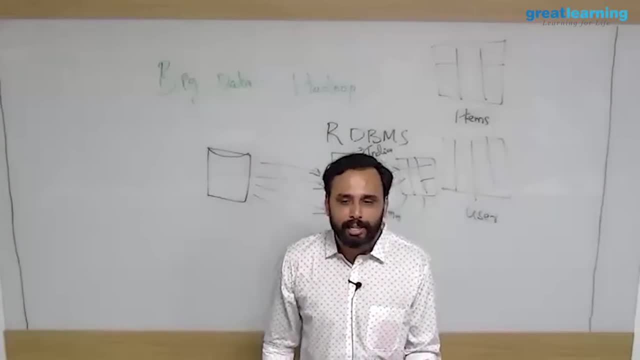 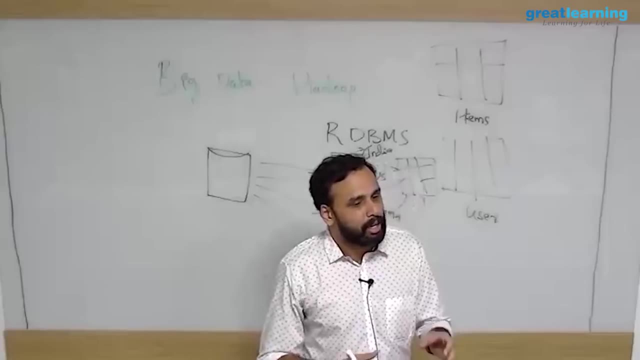 query. the query will take a lot of time. So what I do? I say that, okay, don't store the full table, divide the table or partition the table. To partition. I will say that I have to use some logic for partitioning. I cannot physically divide the data, That's. 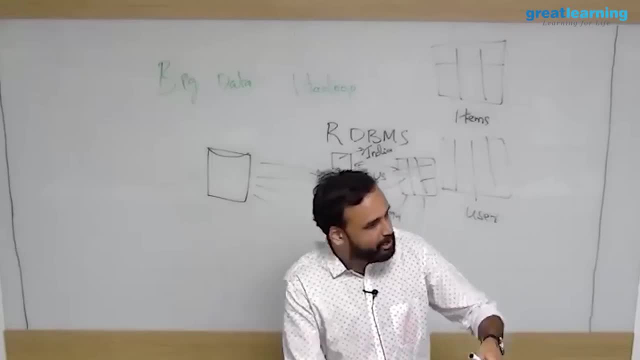 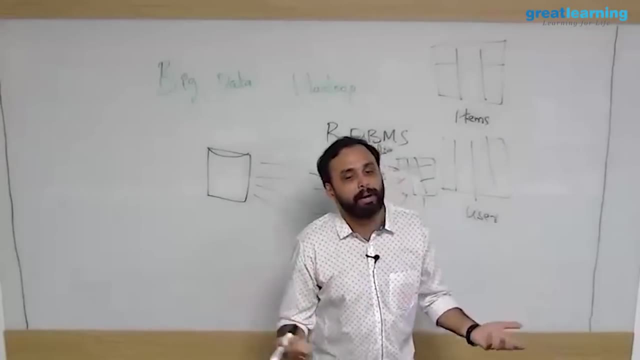 not possible in RDBMS. I cannot say that take a table and cut it into four Doesn't work, So I have to logically partition. So I have to say that there is a country column. How many countries are there in the world? Maximum, 155, right? I'm not much of a geography person. 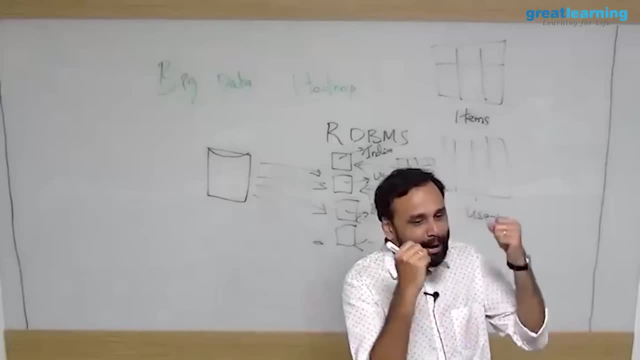 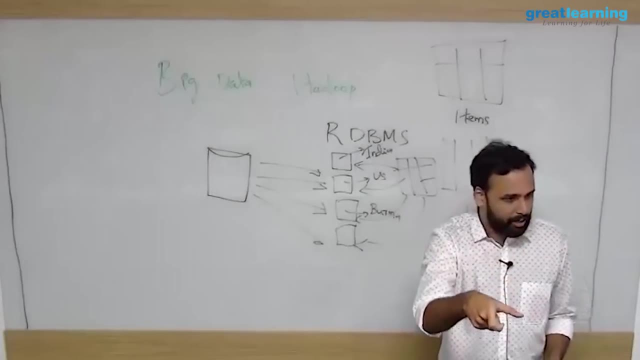 but I think somewhere around 155,. right, But at least people who buy iPhone, 155 countries are there. So I will say: take the country column, So everybody who is buying an iPhone based on the country column, it will partition your data. right Now I have four boxes This. 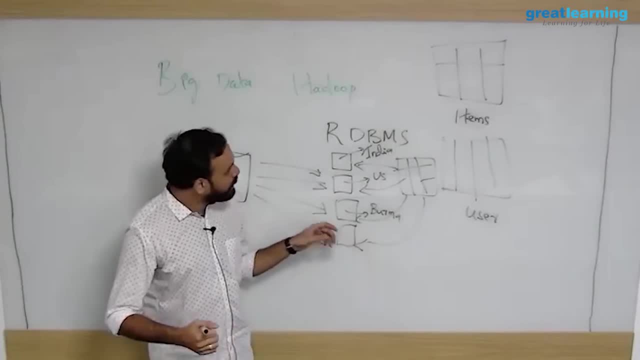 box has India data, US data, Burma data and something data- Again. same story. If you're running the join query, this box has to process all the India data for join query. This box will complete very fast. This guy has to wait, So again you're so. the problem is that traditionally, 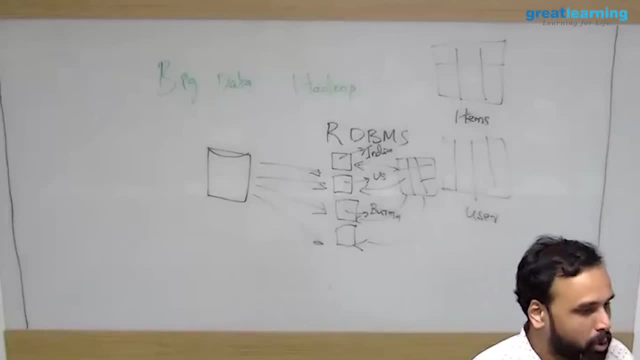 people were using RDBMS systems and data warehouses to store the data. Now what is the drawback? One of the drawback is that, as they started to use RDBMS and data warehouses to store the data, now what is the drawback? One of the drawback is that, as they started to use 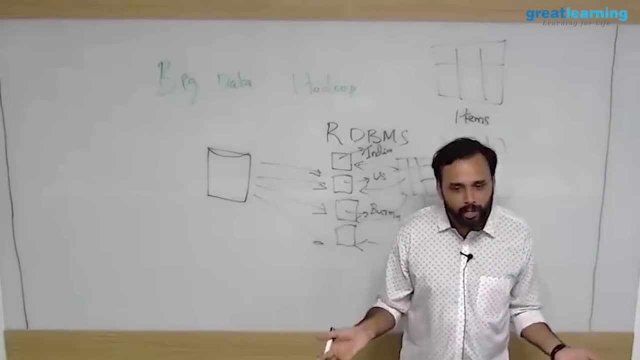 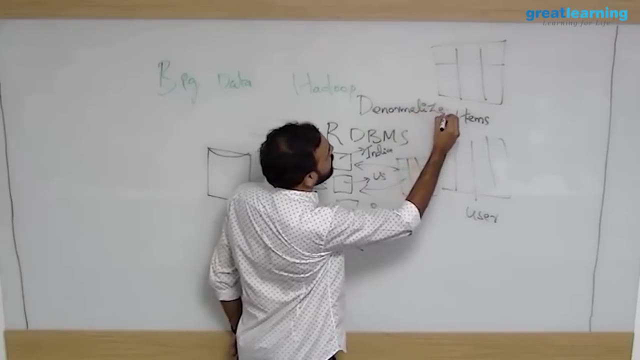 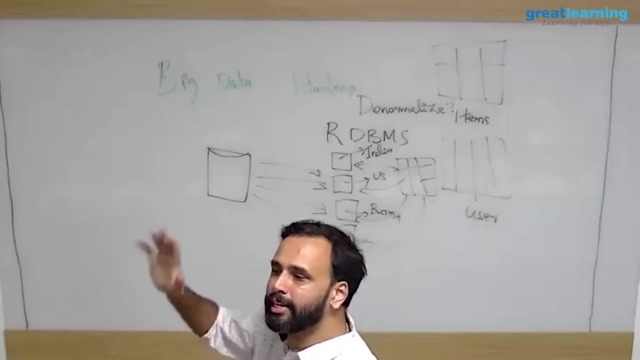 RDBMS and data warehouses to store the data. the size of the data increases, Your processing will become very, very slow. Why don't you denormalize the data? Why don't you denormalize the data? For example, all the transaction data, user data, everything I'll keep in one. 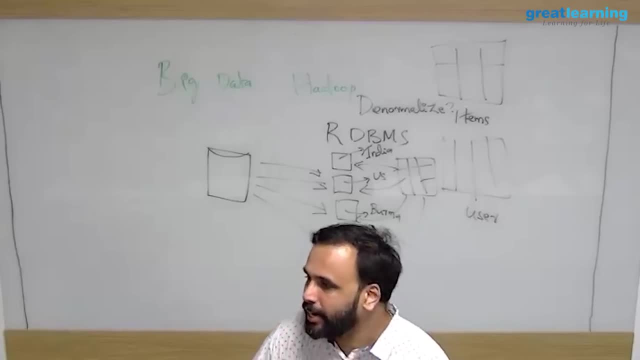 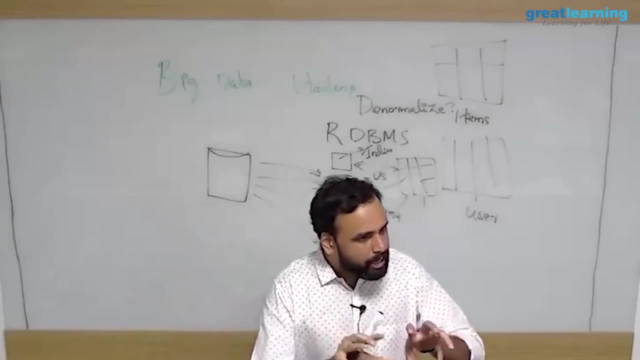 table. Is that possible? I can't do So. that is the reason they don't provide the denormalized solutions. If you look at RDBMS systems, they will always say: normalize your data so that it will be represented in a different way. So the reason is that they don't provide the 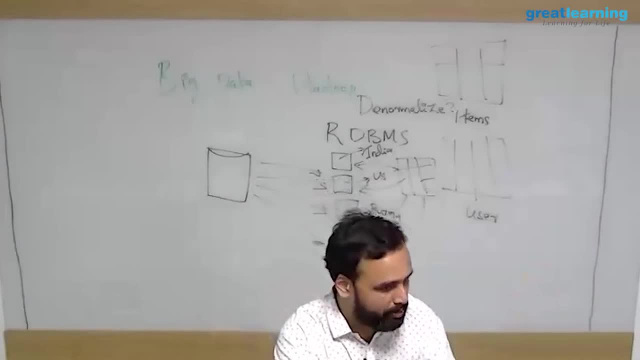 denormalized solutions. If you look at RDBMS systems, they will always say: normalize your in different, different tables and whenever you need the answer, you do a join and you get the result. second drawback: this is only structured data, meaning anything which you can represent. 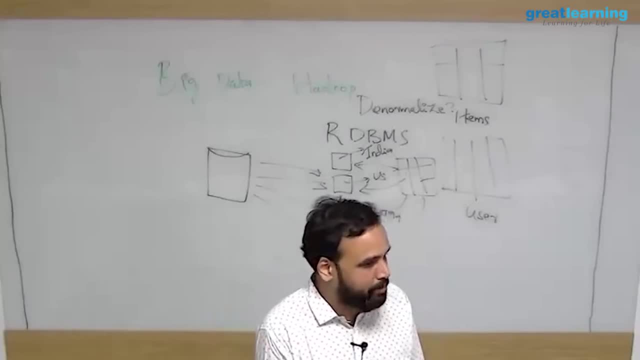 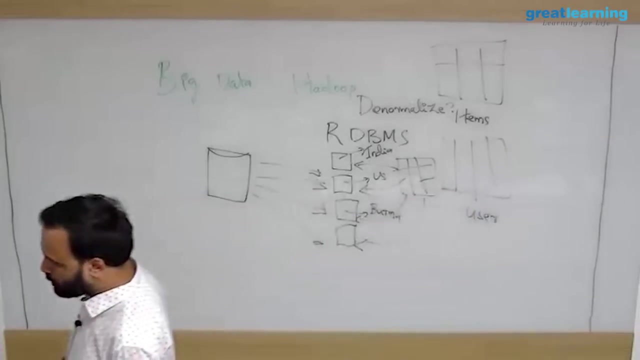 in row column. i can dump here like an excel sheet data, right? can i dump images and audio files in this table, yes or no? can we store unstructured data in rdbms? yes, you can. there is clob blob and all objects right, but can it process unstructured data? not possible. so size of 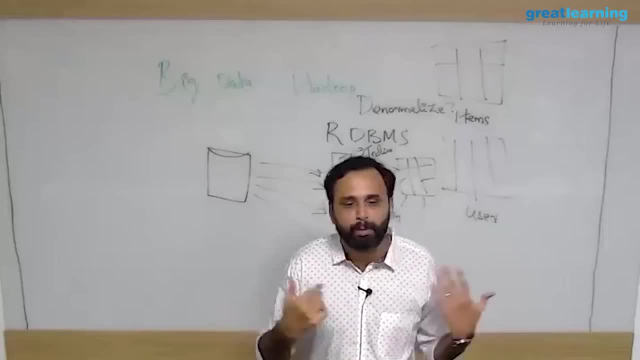 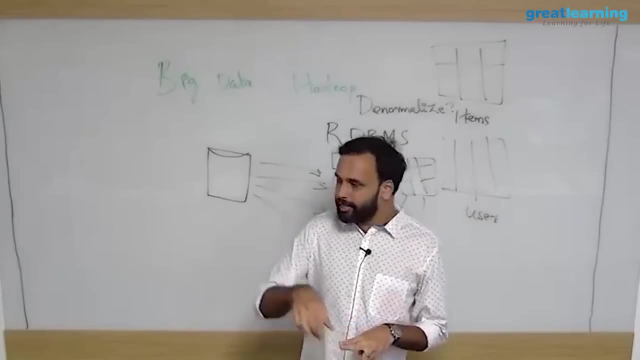 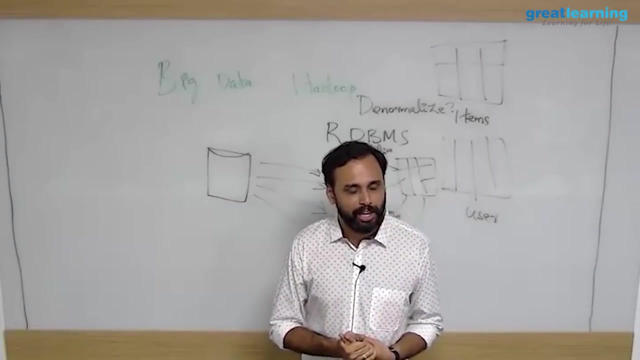 the data increases, it cannot cop up with processing. one of the problem right? second problem is the schema, meaning anything which you can represent in a row column format, i can dump in an rdbms. anything apart from that, i have to figure out a solution. so what is the actual solution? if i have? 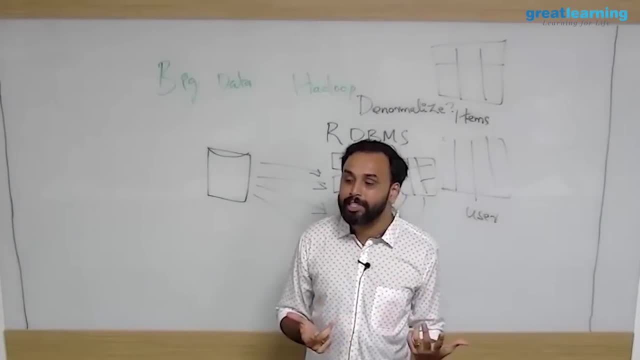 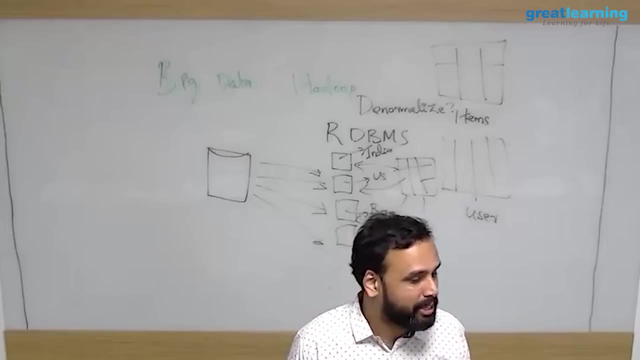 to store images and retrieve them in real time? how does flipkart stores the data? i was working with flipkart for some time. flipkart has around 10 million products. each product has 10 images. that is 1 billion images. so when you click on a iphone x picture, 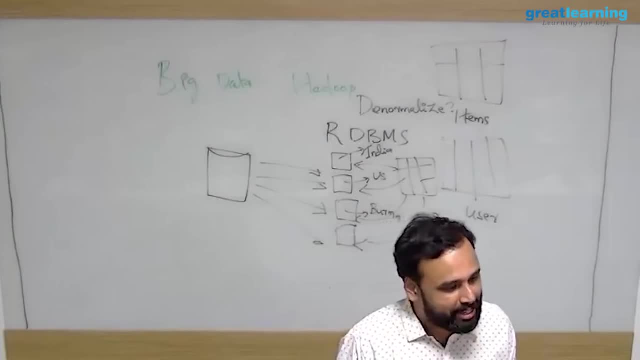 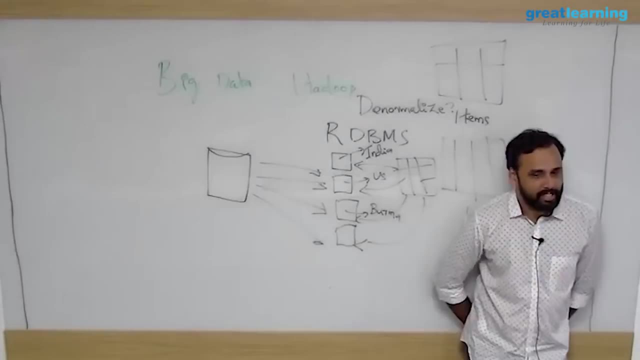 on flipkart. flipkart will say that come after 10 minutes or immediately display. have you ever thought how it is happening? how it is happening, right? so do you think they are dumping in an rdbms and picking it from there? 1 billion images. there is a whole arena of databases called 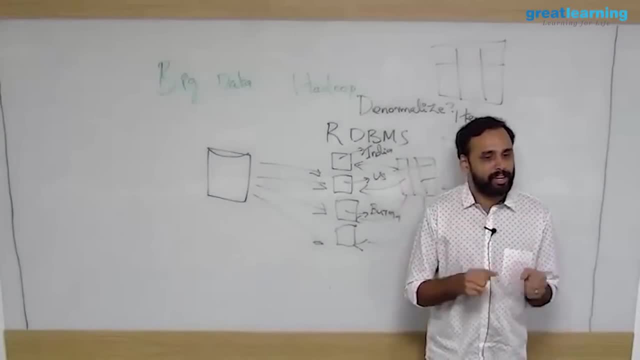 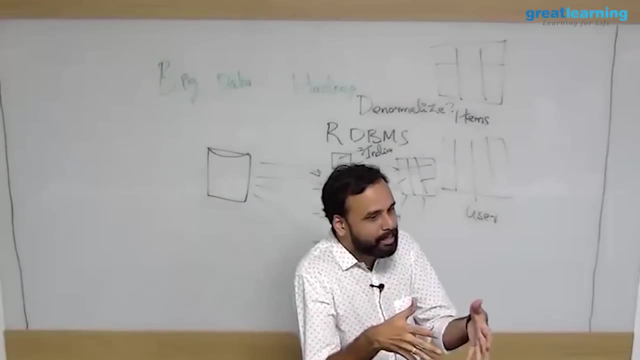 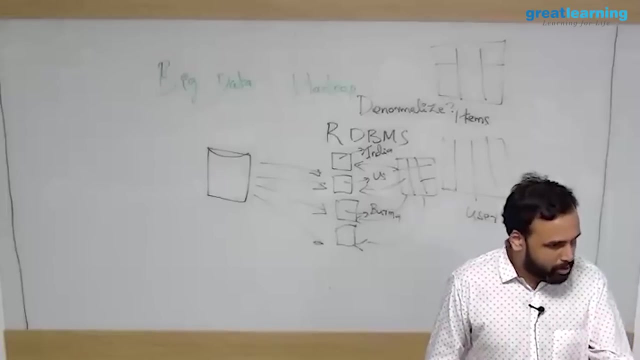 no sql. if you have heard about mongodb, cassandra edge space, neo4j, waldemort, these are all popular vendors of nosql database. so no sql databases will help you to store and retrieve unstructured data at any speed you want. so what amazon, amazoncom, actually does? 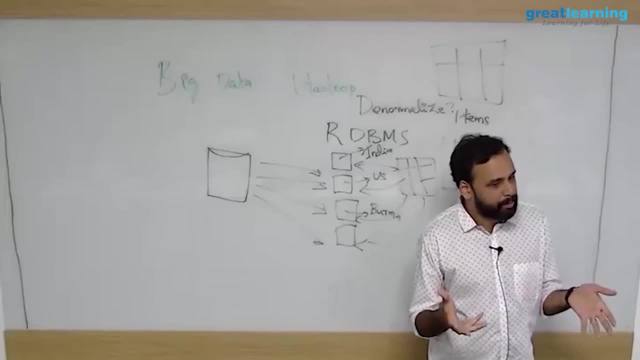 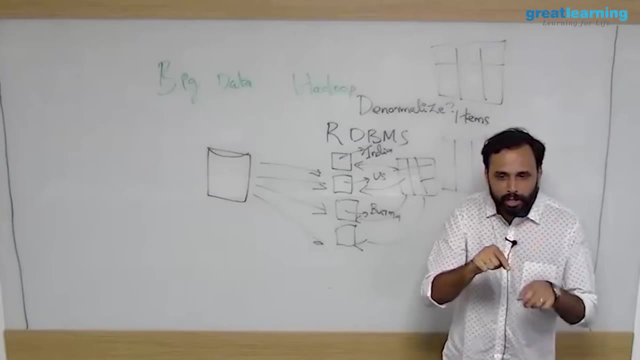 amazon has something called dynamodb. dynamodb is a no sql database, so in dynamodb i don't have a row column, i have key value pairs. so what they do, the key will be the product name. say, you are clicking on iphone x, iphone x is the key. 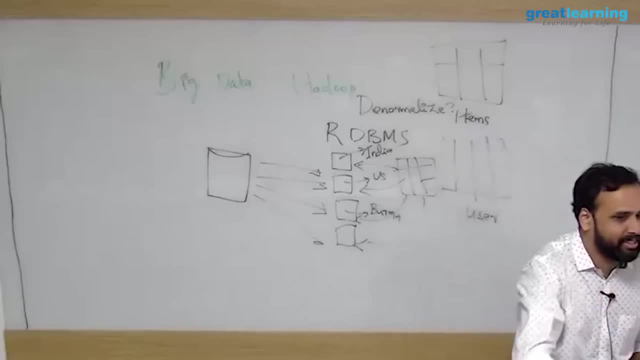 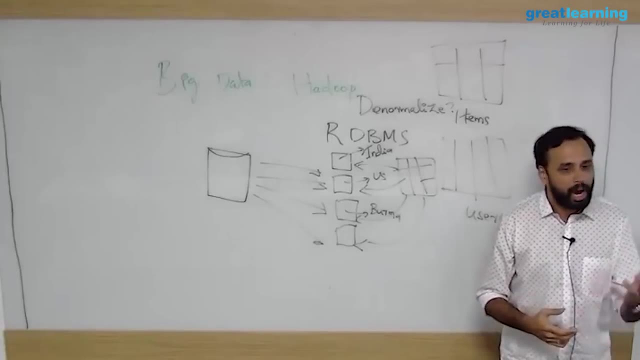 will be all the data you have. So the moment you click, boom, your page is there. So now SQL databases are really faster. Also, it helps you to store unstructured data. How are you booking a cab using Ola? If I try to get a cab using Ola, I open up Ola. 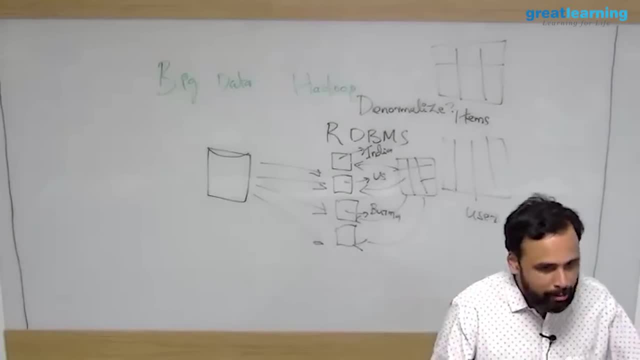 how many customers Ola has- Millions in India, And all of them are booking at the same time, right? Do you think all your requests are taken by an RDBMS and searched in the table and give you a cab? Does it work? 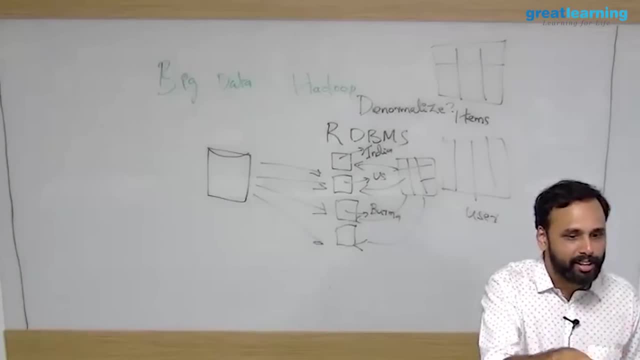 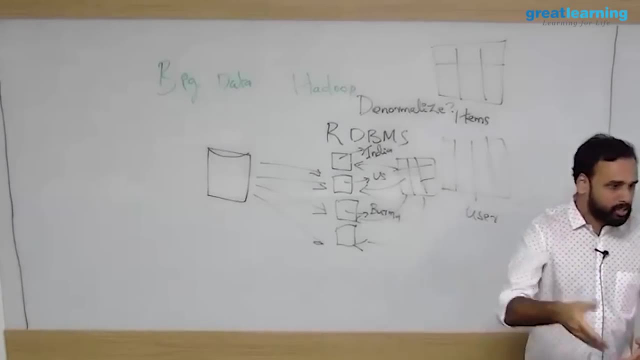 Can an RDBMS system handle 30 million, 40 million concurrent sessions on this amount of data? calculating route? MongoDB: no SQL database. Ola runs on MongoDB. I was working with Ola for one of their design problems actually. 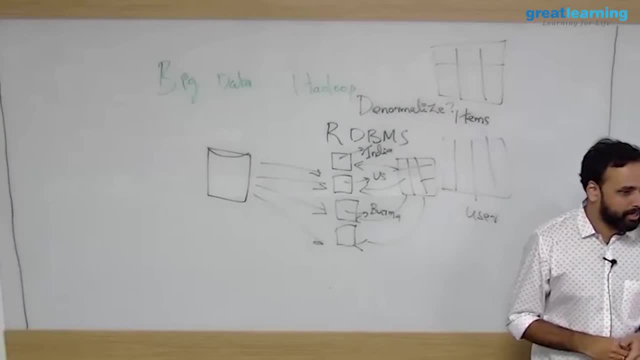 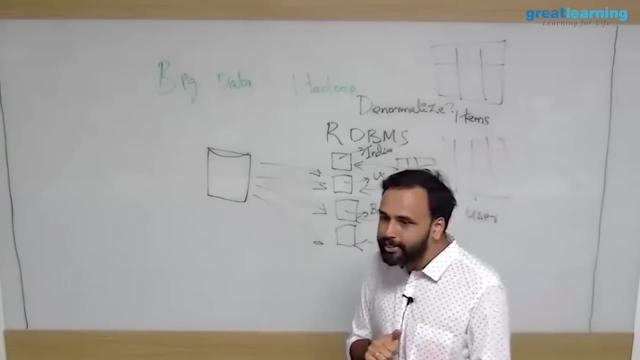 So I didn't design anything, but they told me that they are using MongoDB. So the second drawback of your RDBMS is scalability, is there? Third is price. Price is a problem, right? I mean, obviously, if you calculate the cost. 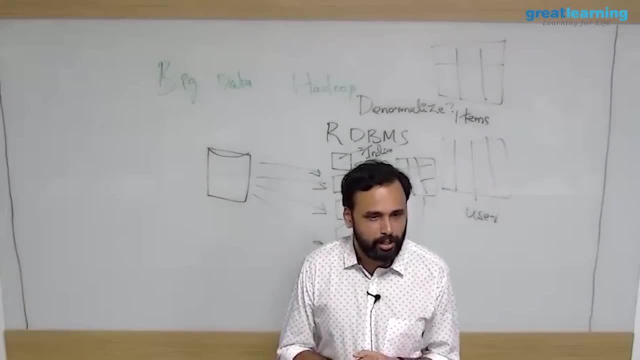 if you look at RDBMS, you can calculate the cost. If you look at Oracle and all, they are very, very costly solutions. Traditionally storing the data on an RDBMS and retrieving is not good for the modern day. 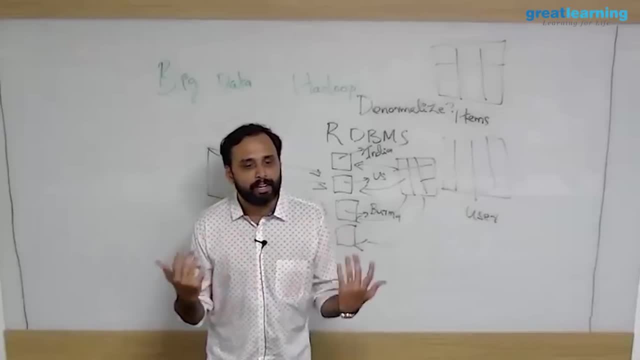 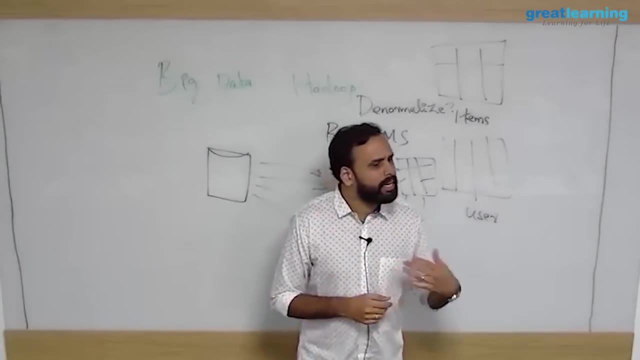 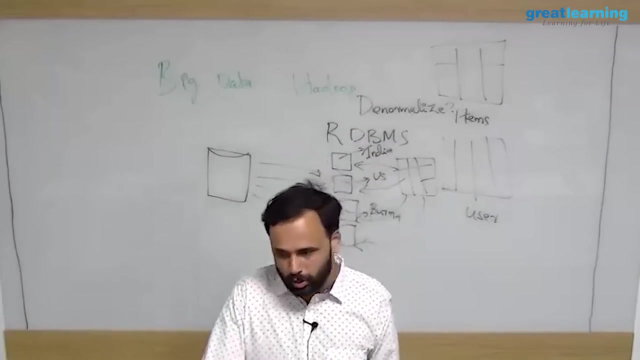 In the modern day, what is happening is that every company wants to collect and analyze the data, Be it banking industry, e-commerce industry or any industry that you want, they want to collect and analyze the data. So, to give you an example, if you visit Amazoncom or Flipkartcom, 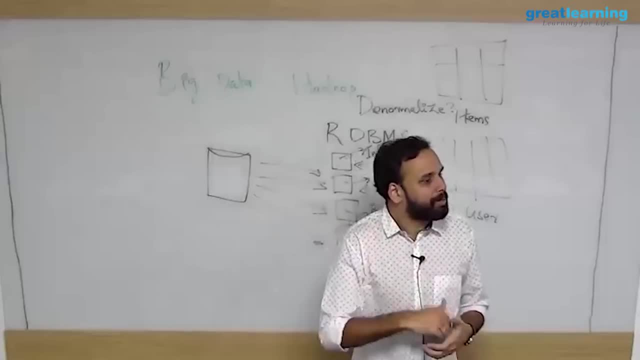 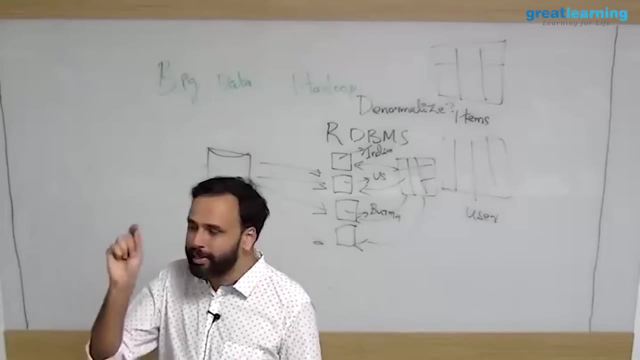 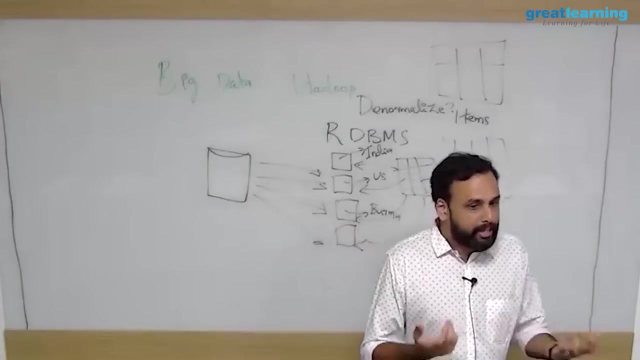 what is happening. They start tracking from which IP address you are visiting the website, how long you are clicking on a page, which items you are adding to cart, which images you are clicking, which offers you are clicking. All this data is analyzed to understand how a customer will behave. 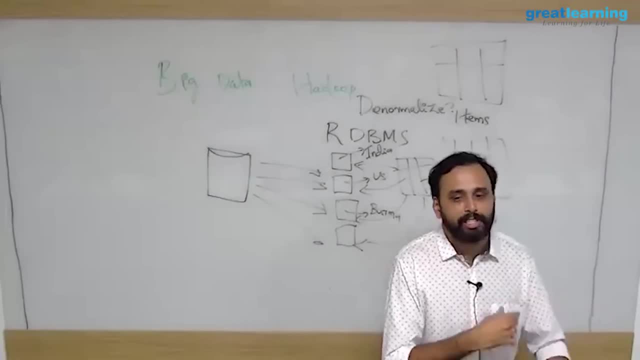 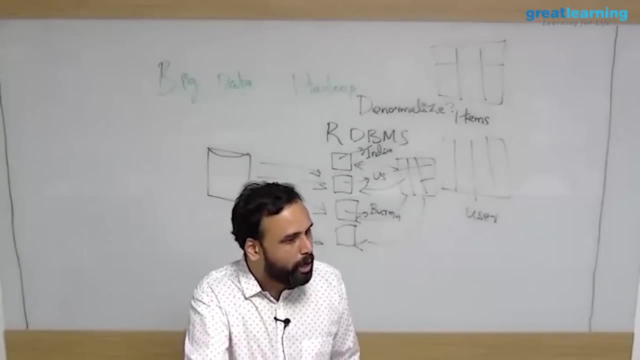 That is how they do marketing right. So the more you start visiting the e-commerce companies, you start seeing recommendations, and all the more The more you visit Amazon, they will start recommending products to you, asking you to buy. So they have to collect all this data. 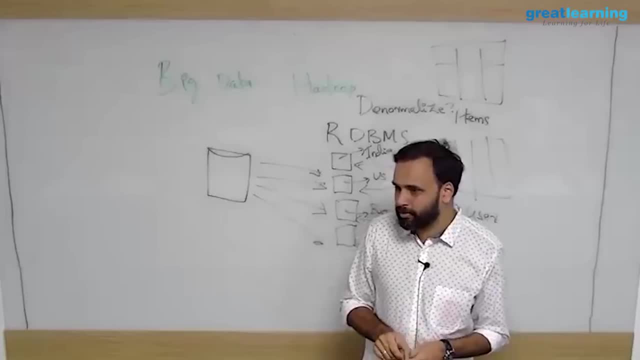 So when I was working with Flipkart, Flipkart said that they collect data from the apps that you are using, from the website that you are having, even from social media. Flipkart is very active in social media like Facebook, Twitter, all these places they are active. 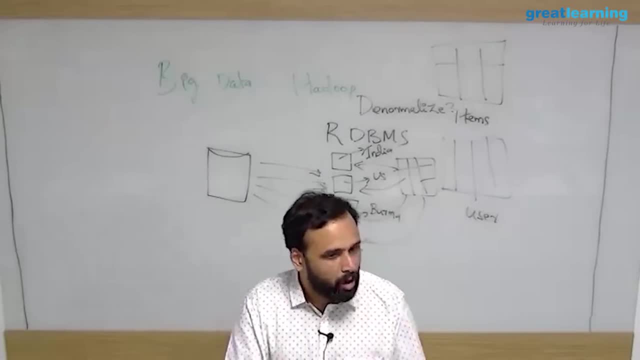 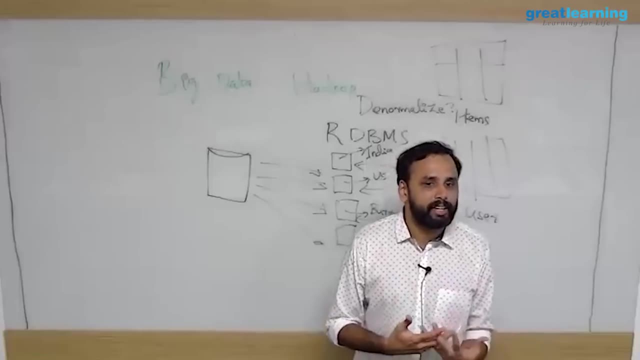 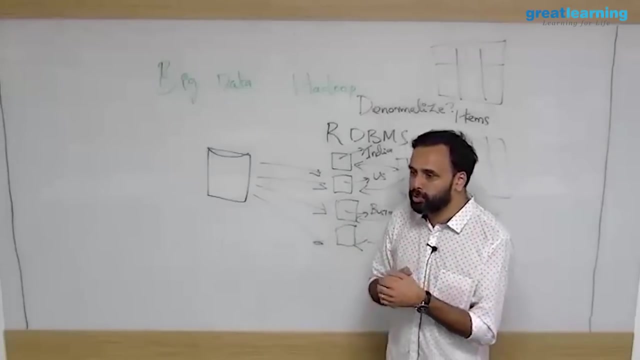 So if anybody tweets about Flipkart or visit their Facebook page, all this data is being collected. Now this is actually called big data. So the technical definition of big data is this huge amount of data which you cannot process using your traditional methods. 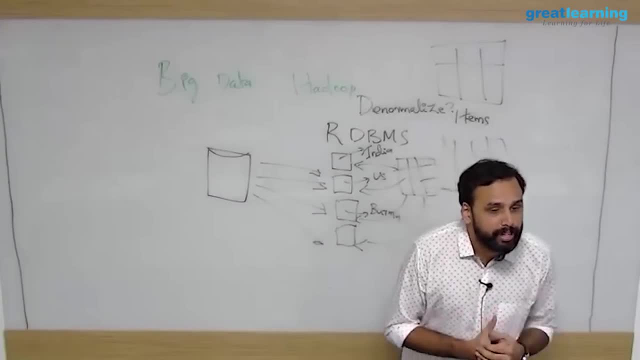 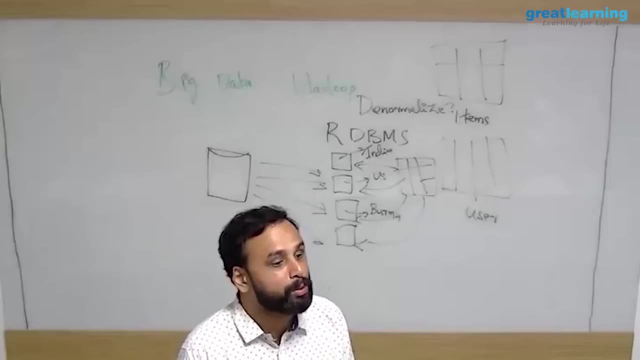 That is called big data, right? So why that is of interest to us. we are going to figure out how to store this data- huge amount of data, right- and how to process this data. When I say NoSQL, databases are there. 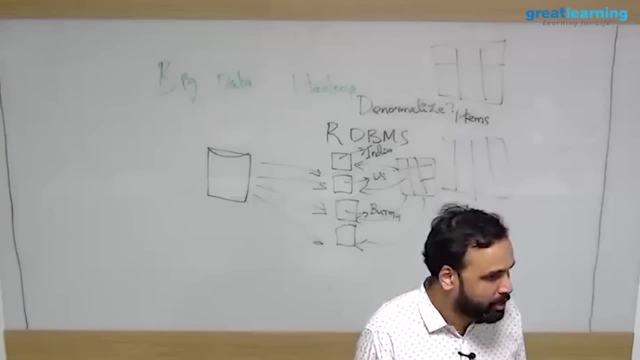 it does not mean your RDBMS is gone. So many people ask this question. OK, RDBMS is the only solution for transaction management. So, even if you're buying something from Flipkart, who will complete your transaction? Oracle, probably, or any transactional system. 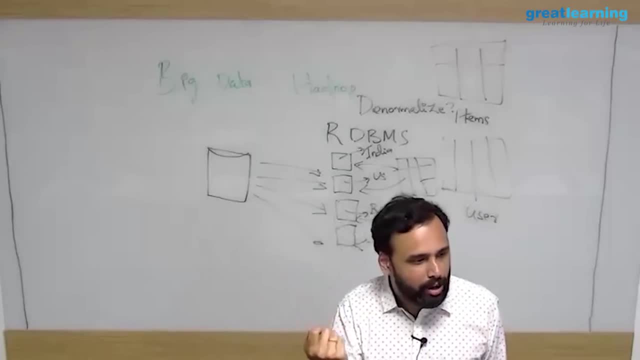 For transactional management. and why is that? Because RDBMS systems are the only ones which can ensure the ACID properties right, If a transaction goes or not goes. You bought something from Flipkart. tomorrow, Flipkart cannot come back to you and say that.